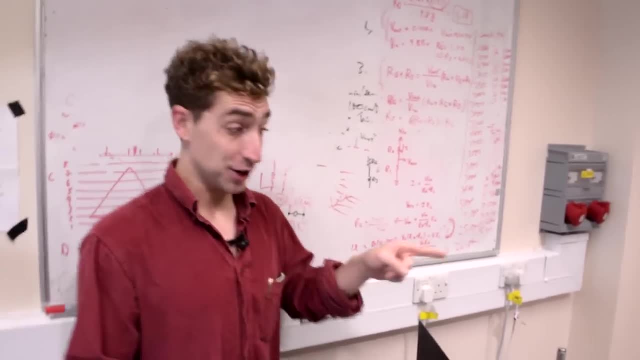 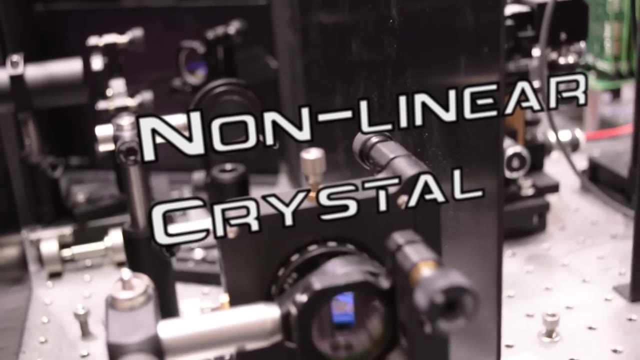 a process whereby one photon splits into two. So I can show you how we do that over here. All right, because we get a big laser beam. we fire it at this crystal. So there's a special type of non-linear crystal. When you put light into non-linear materials, weird things happen. 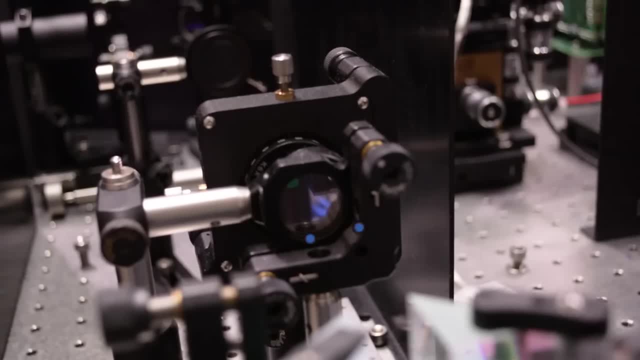 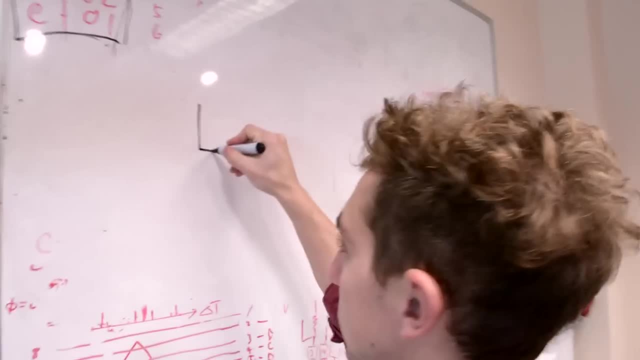 okay, And in this particular one, two photons pop up. So what are the important laws of physics? All right, well, there's conservation of energy and there's conservation of momentum. So imagine this crystal, this non-linear crystal, and I'm going to fire a photon in it and it's. 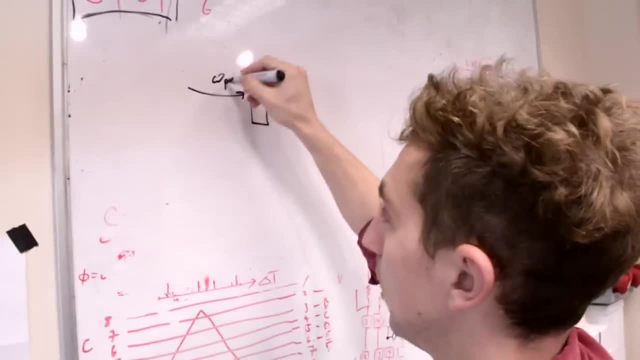 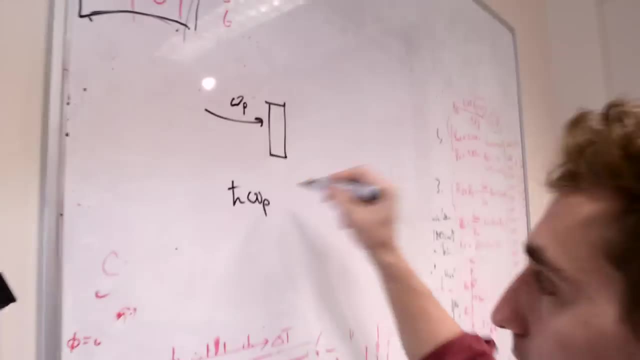 got some frequency, all right. It's got some wavelength And that's going to be a quantum wave. That tells you about its energy. okay, So its energy is an H-bar over gas And then two photons are going to pop up, that guy and that guy. Call them number one and number 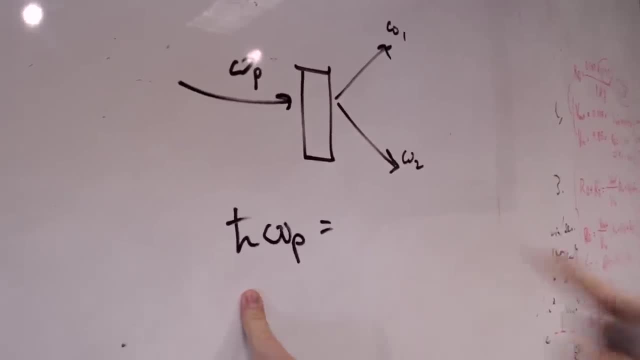 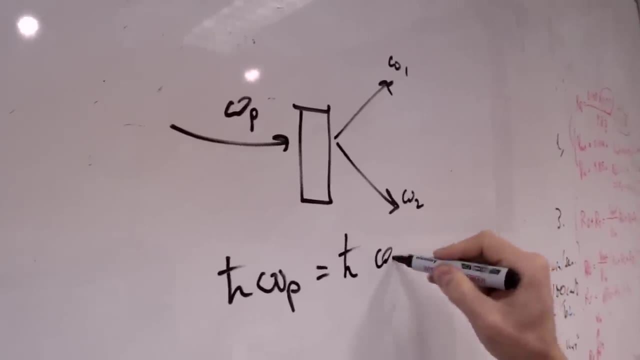 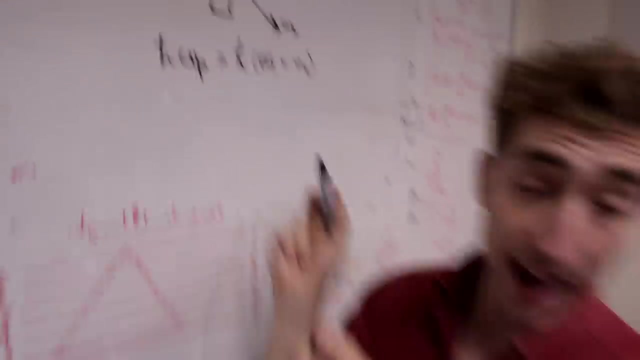 two, And we know that energy falls with equal energy afterwards. so the energy of these guys must add up to the energy of this guy. So the frequency of these guys is half the frequency of that one. okay, So that tells you about the energy of this photon. It tells 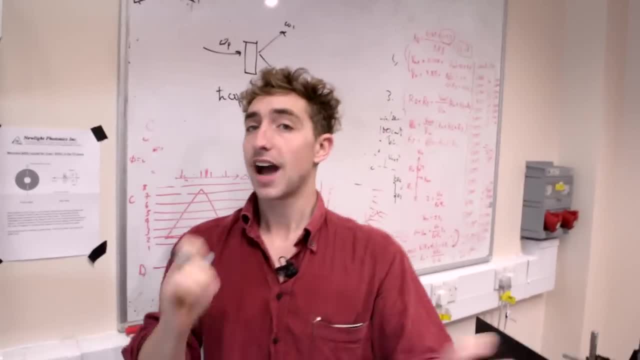 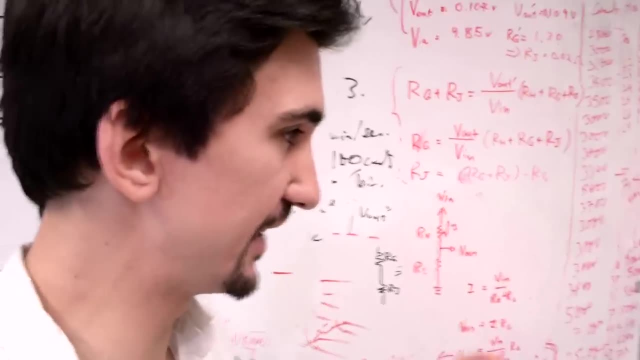 you what the wavelength is. So we pump it with 400 nanometre light and the photons that come off are 800 nanometres. Okay, so you send a beam of light into this non-linear crystal and each photon that comes in then produces two photons coming out of it. 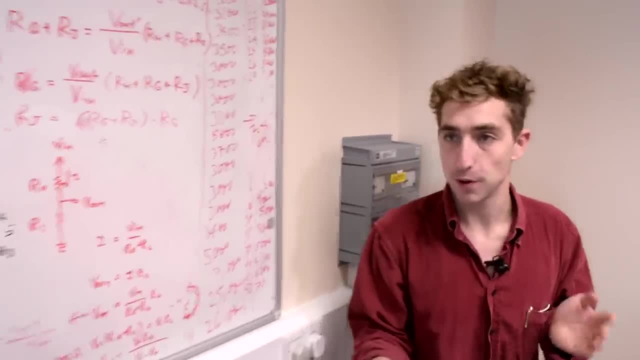 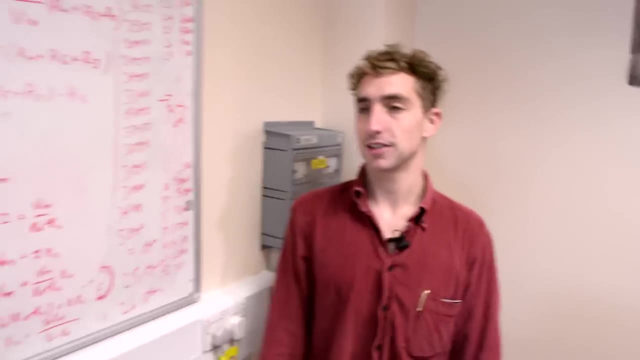 Not each one, some of them. There's a very small probability it's going to happen. But because we've got a big laser that's got trillions of photons in it, you know you can make that probability appreciable. So we see lots of photons. 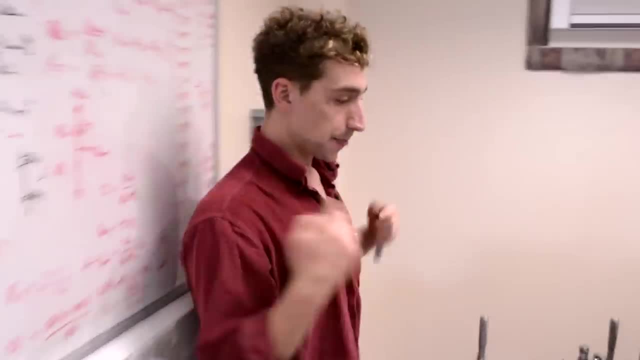 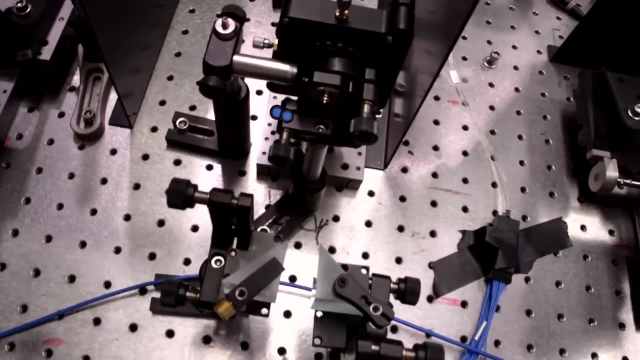 Conservation of momentum. right, That's also very important. So if you look around here, all right, our input, Our input, photon is moving that way. okay, So what we don't want to have is two photons coming off here. That's really bad. Physics doesn't like that. So that's actually why. 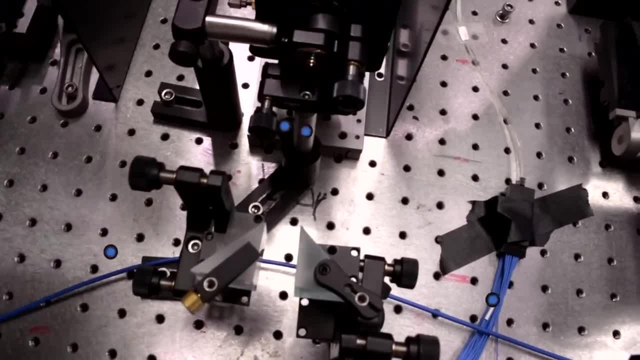 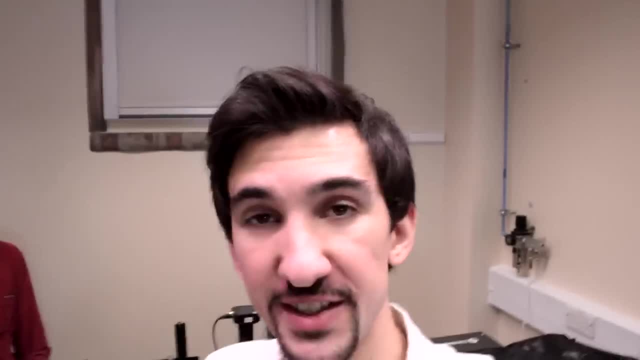 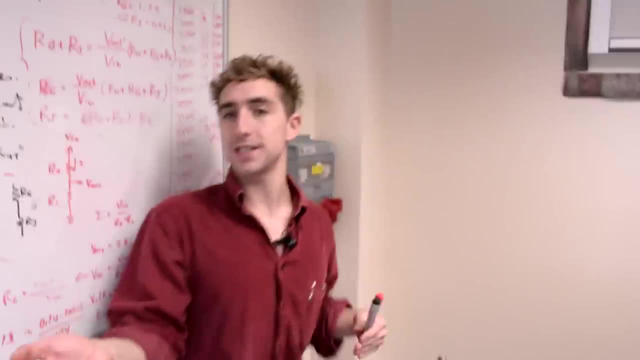 we've got two prisms bouncing right off here. The photons come off like that. So at this point we've made our two photons by sending in this light into this crystal. Is this entanglement? Have we done it? Not quite yet. It's not quite the useful entanglement that we need to do, something like build a. 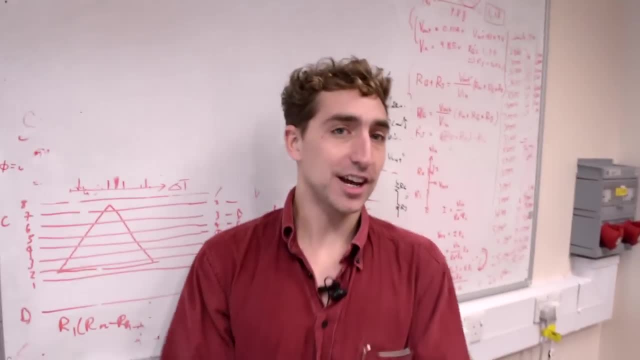 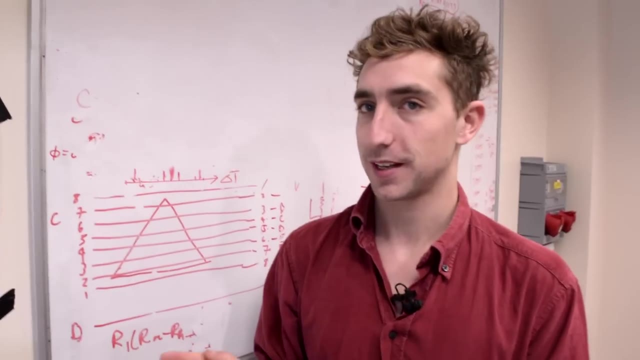 quantum computer. A quantum computer, okay, Because to understand how you do that, you really need to know something a little bit more about this crystal, just a little bit. And the crystals care about polarisation- okay, They care about the way the light moves inside it. all right. So if 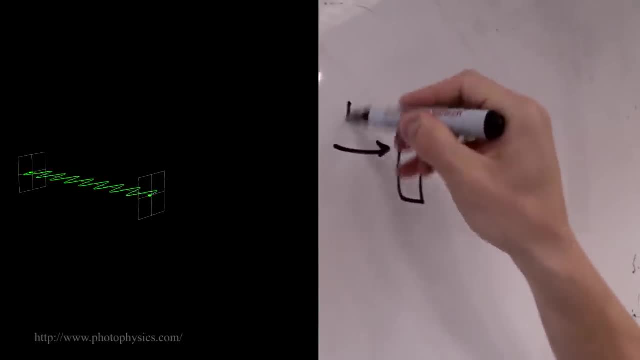 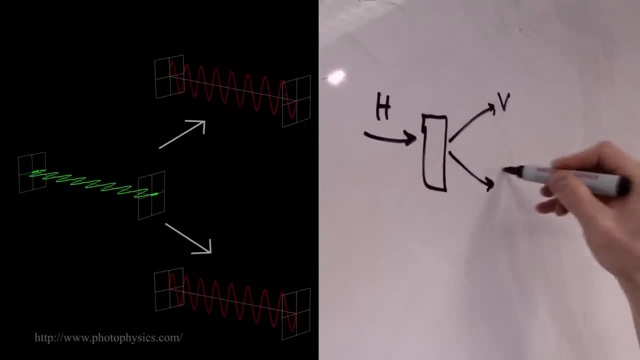 I imagine I get a crystal. If I input horizontal light, the H, the photons that come out are going to be vertically polarised, So this is one type of crystal. I'm going to call this number one What I can also do. 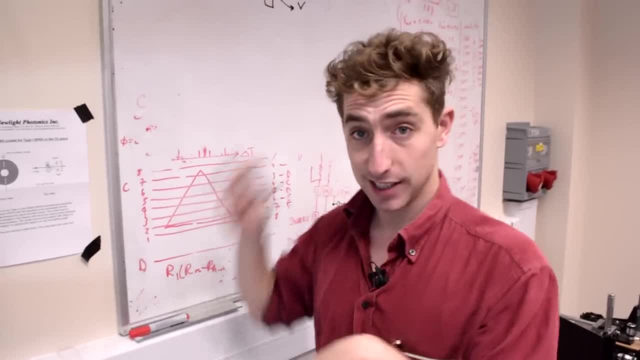 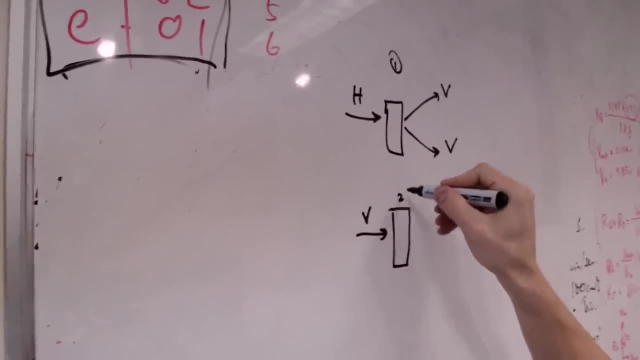 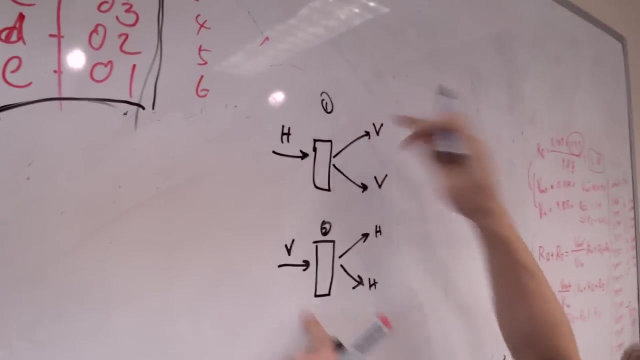 is: rotate this guy by 90 degrees. okay, Just take the same one and rotate it by 90 degrees, such that if I input vertical light, okay, the photons that come off will be horizontally polarised. You get one of these and one of these. put them up next to each other, okay. 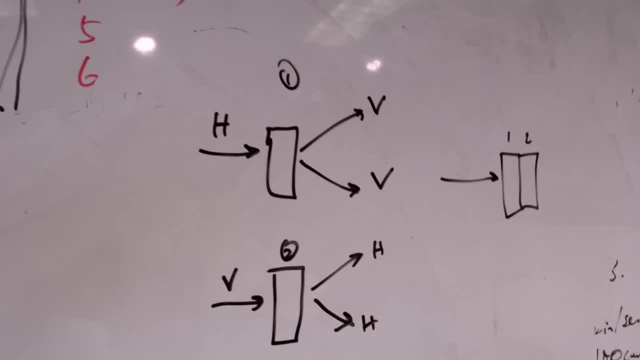 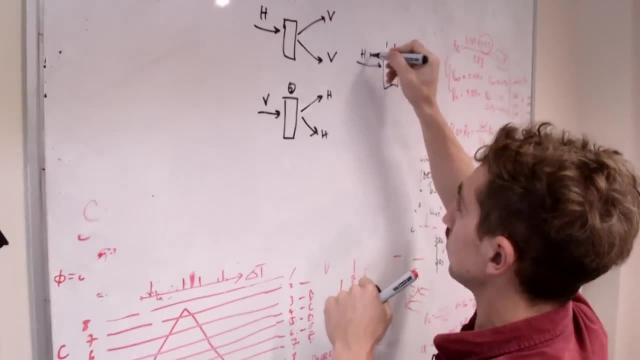 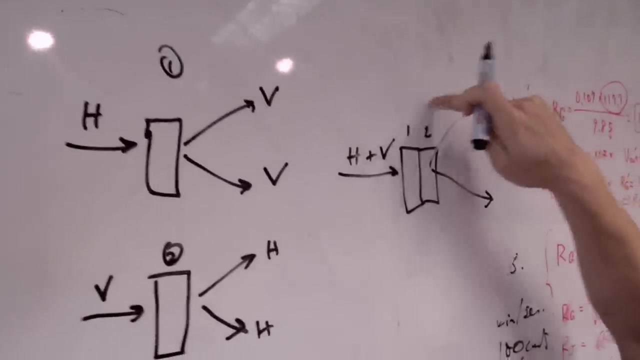 Crystal one, crystal two and you input what we call diagonal light. okay, Diagonal is a mixture of horizontal and vertical, And if you get photons come out, you don't know whether they were created in the first crystal or the second crystal. okay, So you've got to say it's either horizontal or vertical. 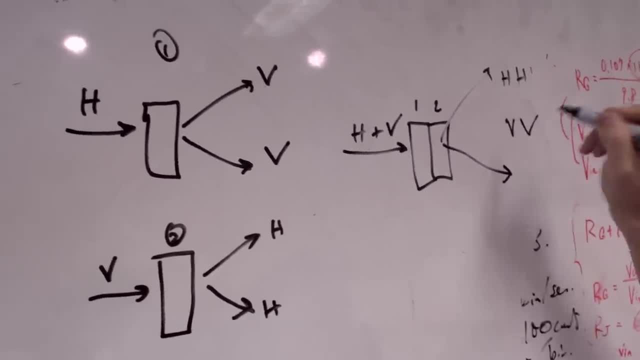 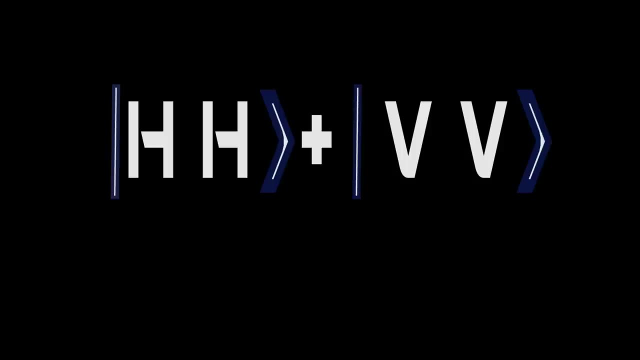 okay, And that is an entangled state. So my question is: why can I not just try harder and work out which crystal my photon was actually going through? Isn't there some measurement I can do? that just tells me and makes this just a question. 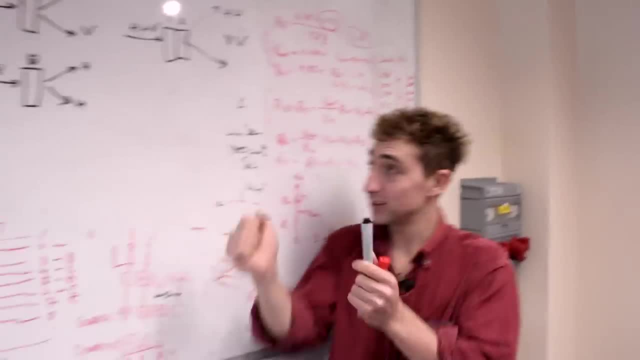 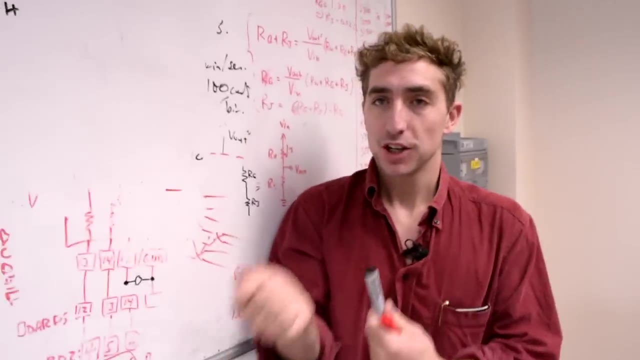 It's a question of uncertainty as opposed to a question of entanglement. No, no, this is quantum physics. okay, This is quantum physics. We're dealing with things with photons, okay. Now, in this quantum regime, you have things that are superpositions, right? 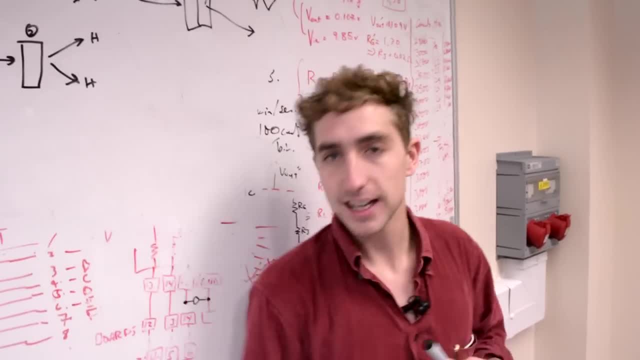 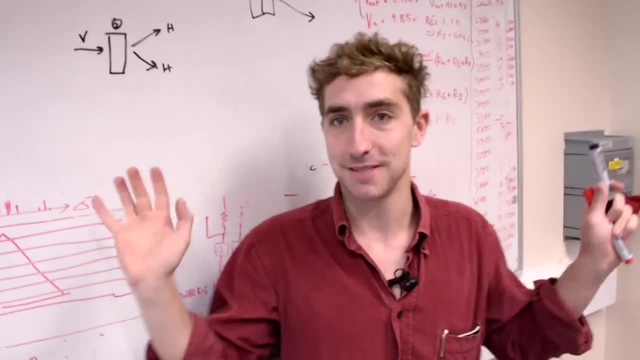 And this is a superposition. Imagine you've got a coin. okay, If I take a coin out of my pocket and flip it right- a coin in our classical macroscopic world. in principle, I could pause time and reality and I could work out the momenta of every little bit of. 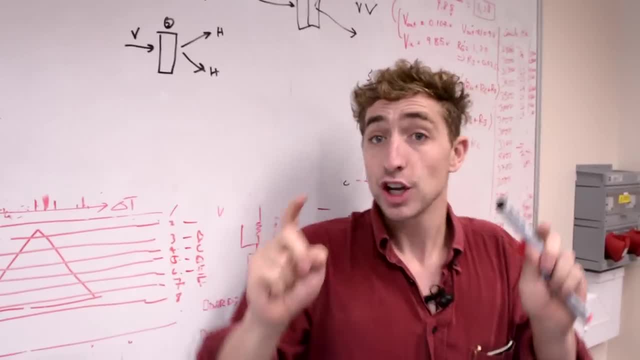 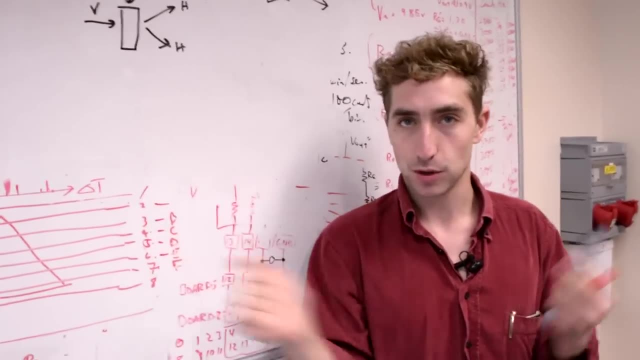 the coin and I could work out the air currents that are moving around, Okay, And I could definitely say whether it's going to be heads or tails. That's, in principle, possible too. it's just really hard. But with a quantum coin, with a quantum superposition, 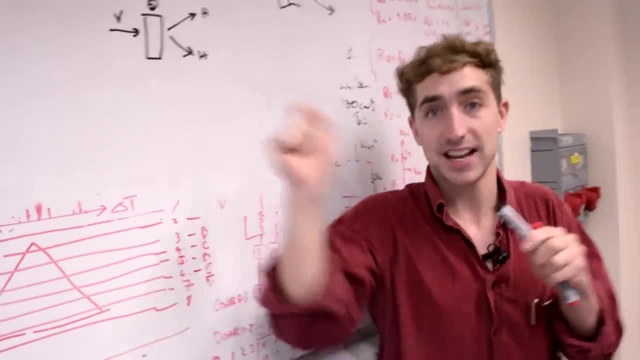 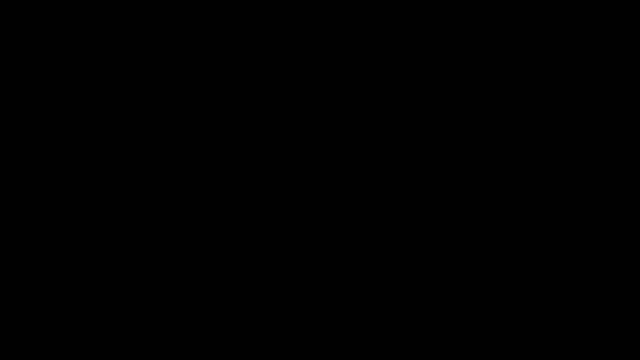 you can't ever know. It doesn't make sense to say whether it's going to be H or V, heads or tails, And that's the situation we've got here. So last week we saw abstractly what entanglement is. This week we tried to get a more practical 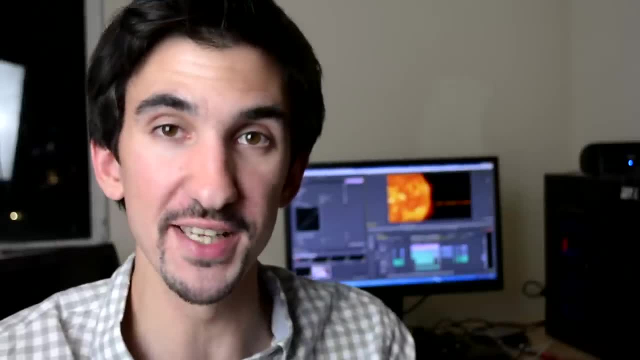 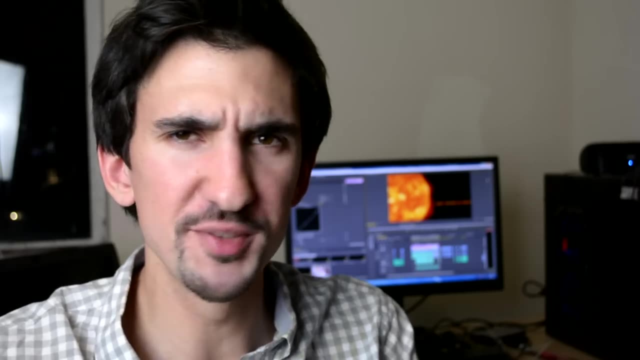 idea of what it actually means to create quantum physics. We did this because I wanted to debunk some of that idea that entanglement or quantum things in general are spooky because they're not. What quantum mechanics comes down to is that there is some physical process which is occurring. 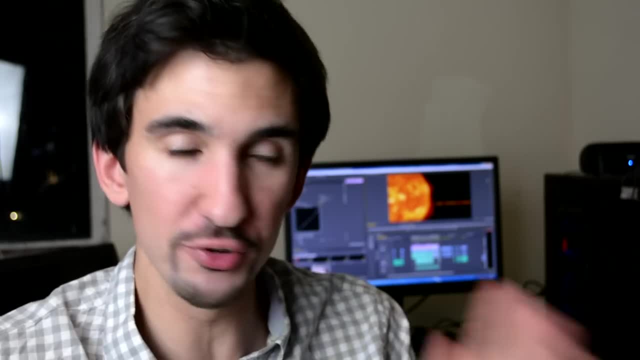 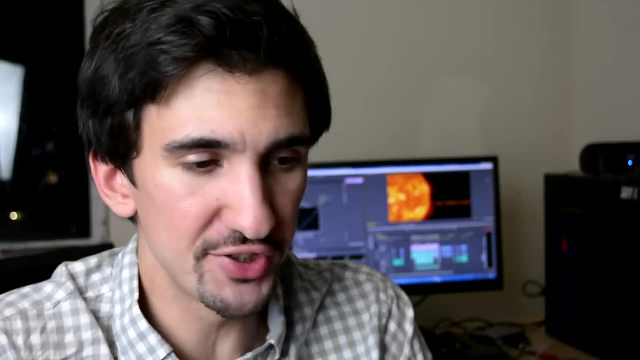 and you can't know what it is Because, as we saw last week, as soon as you go to try and take a measurement on it, it affects the system. It's no longer that same state Now, when you've created two particles which come from a common source and both have this. 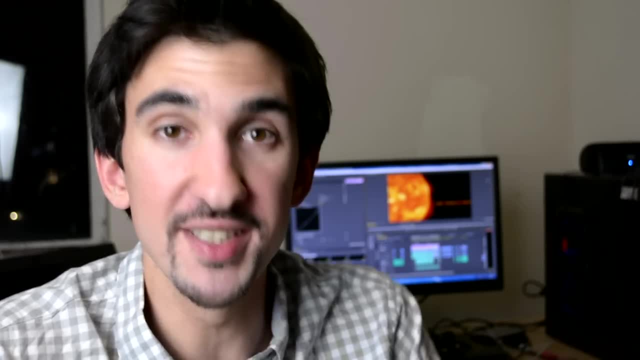 sort of quantum veil about them. you have to think of them in a different way. You can't see them. You have to think of them as entangled. Now, what this means is that, to understand what's happening to one of these photons, you 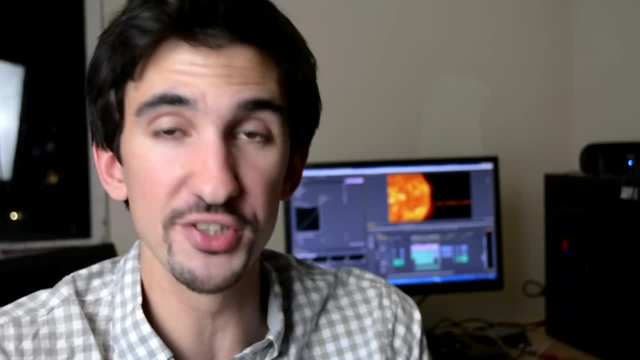 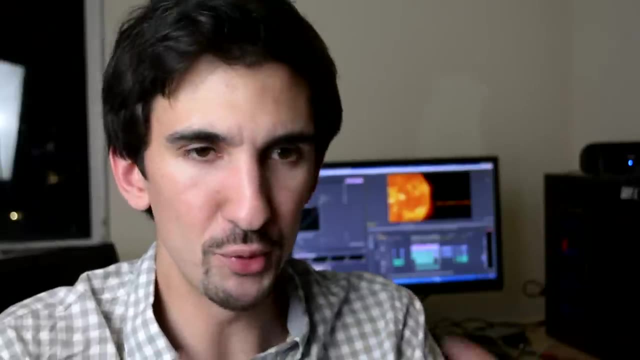 need to consider the entire system. You need to consider both photons regardless of how far apart they are. Now, it's precisely because they are a single system that measurement on one will affect the other, And people will call it weird, because this idea of a space-separated system doesn't. 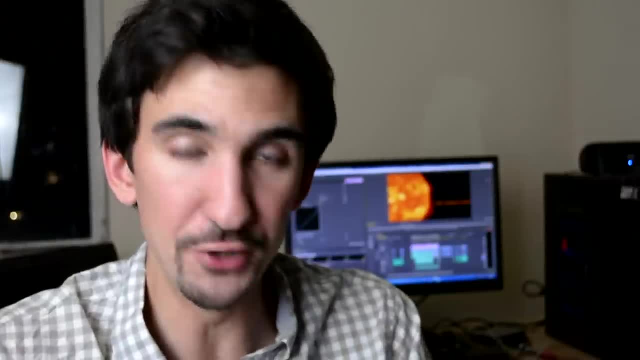 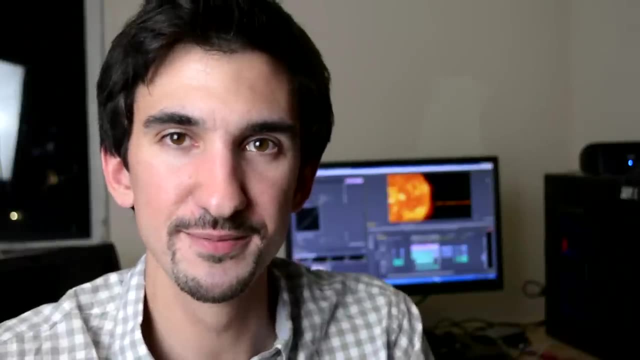 happen in classical mechanics. The quantum veil only exists in quantum mechanics, The idea that you can't see what's happening, so you must account for everything. Okay, guys, well, I hope you enjoyed that. It was just a sort of slightly different look. 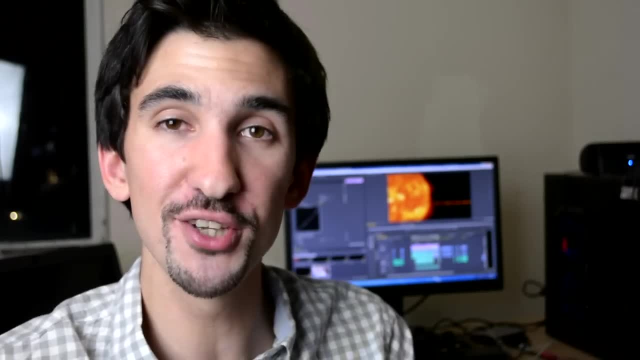 at quantum entanglement than I hoped you were used to. If you like this sort of video, then do consider subscribing to the channel. The link is over there, And if you have any sort of feedback, then definitely leave it in the comments section below. I always read everything. 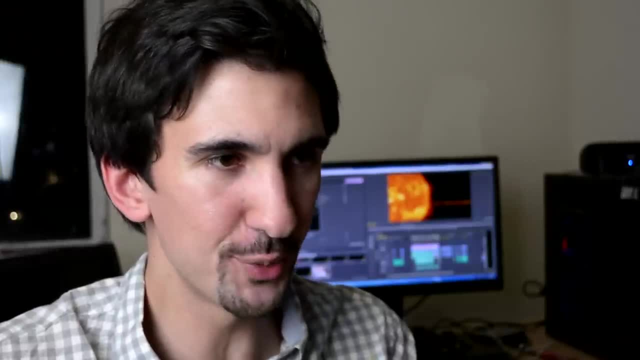 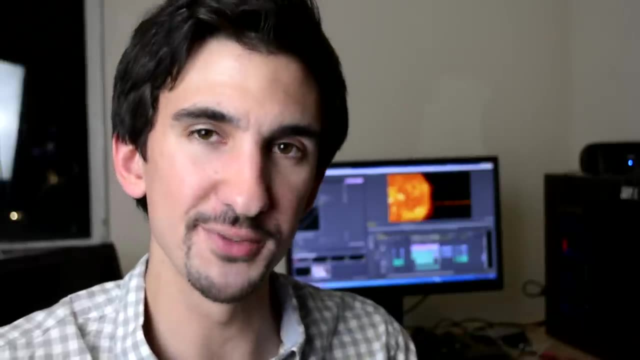 that's put there. I'm actually off to America for a few weeks, so I'm not entirely sure about what I'm going to do about putting up videos, but I will do my best. But anyway, most important thing, have a lovely week And I will see you hopefully next week. Bye. Captions by GetTranscribedcom.